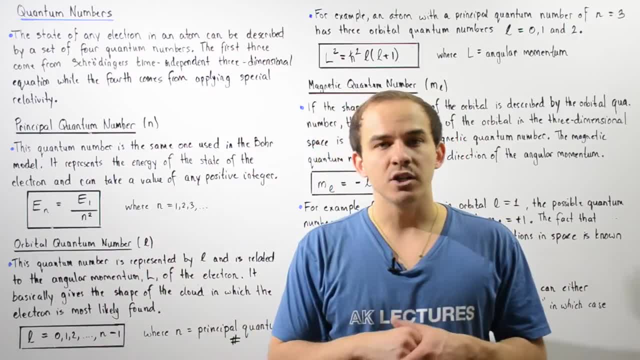 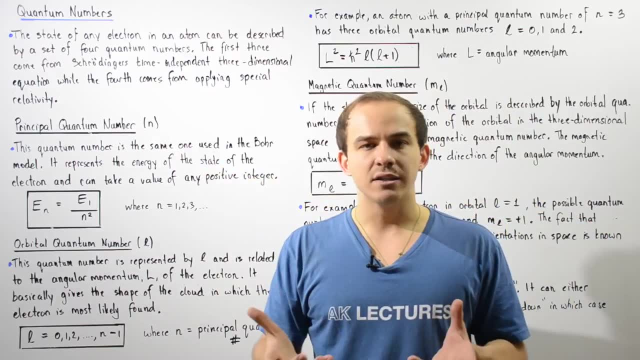 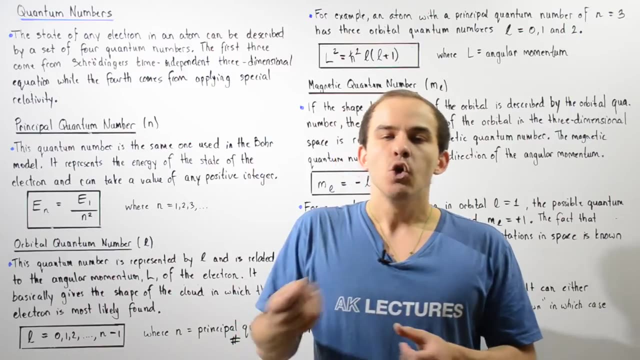 azimuthal quantum number or the orbital quantum number. And the orbital quantum number is given by lowercase l, And the orbital quantum number is related to the angular momentum given by the uppercase L of the electron within that atom. Now, what exactly is the meaning behind the orbital 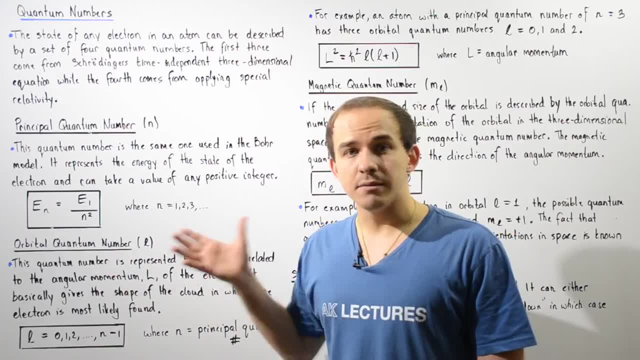 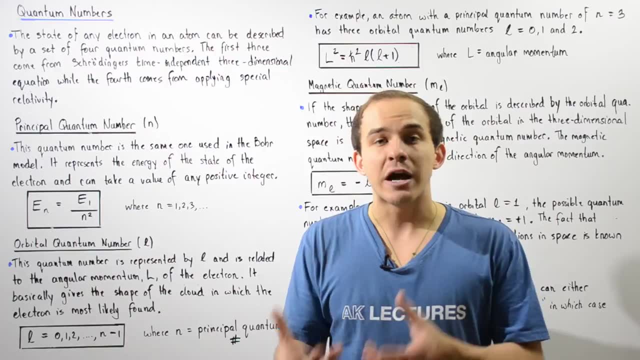 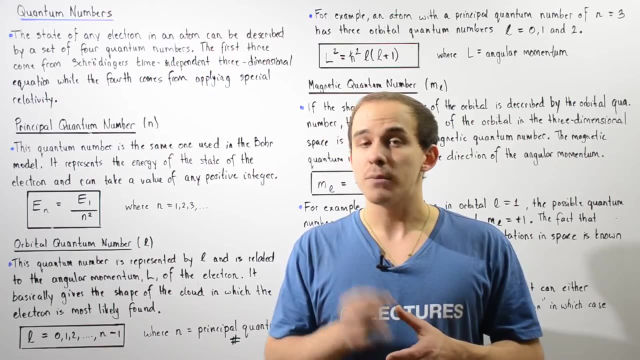 quantum number. So basically, the orbital quantum number describes the shape and the size of our orbit that we're dealing with. It describes the shape and the size of the electron cloud that is produced by that electron. Remember, the electron cloud basically gives us the shape and the size of 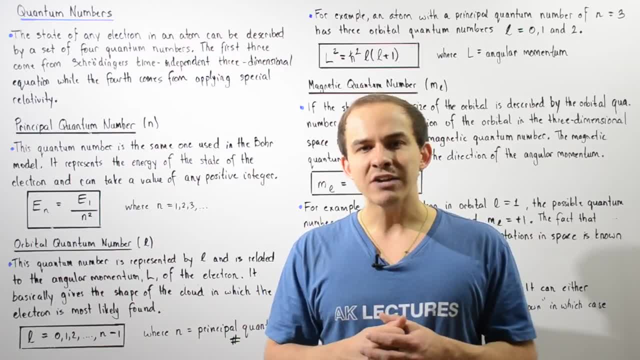 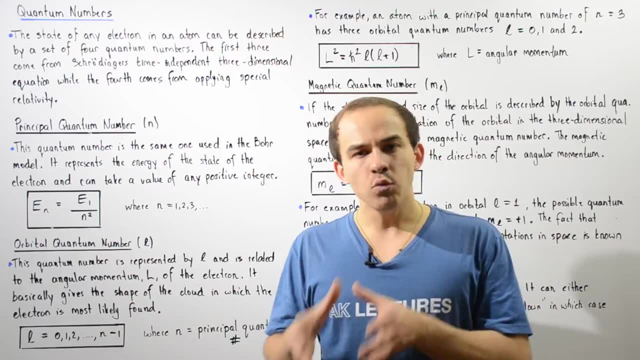 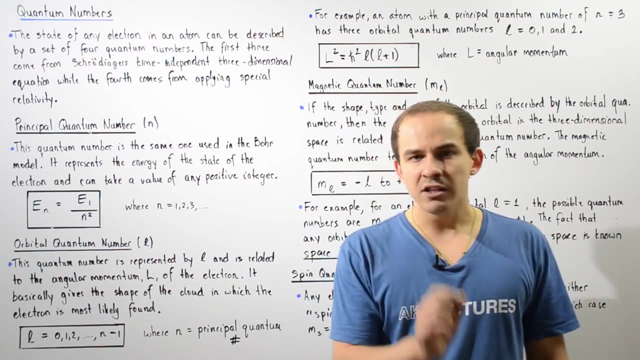 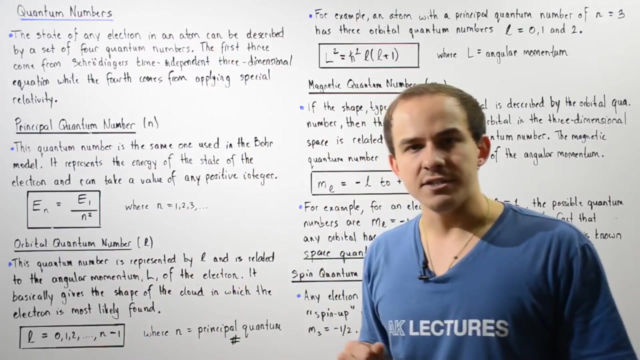 the most probable location of our electron within our atom. So it gives us the shape of the most probable location in which our electron is actually found around that atom. Now, what exactly are the values that the orbital quantum number can take? Well, L is readily given by this equation. So 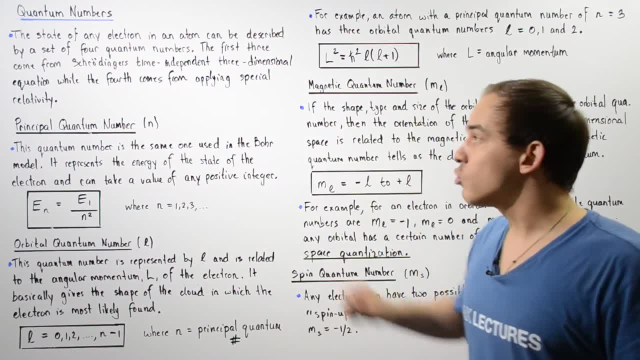 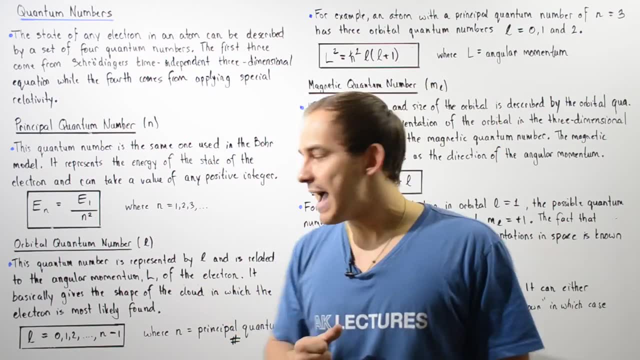 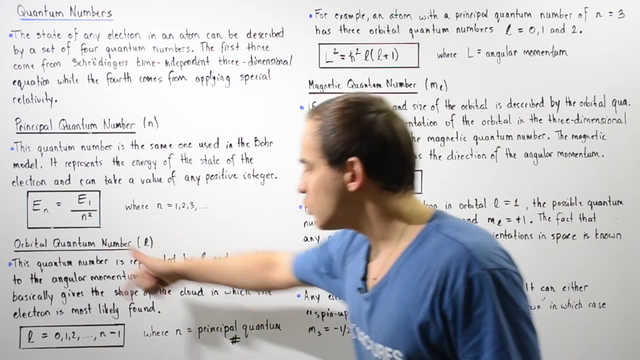 basically, if we know what the principal quantum number, n, is, we can determine the number of orbitals that our atom has. So L is equal to 0,, 1,, 2,, 3,, 4, and all the way up to n minus 1, where, once again, n is the principal quantum number. For example: 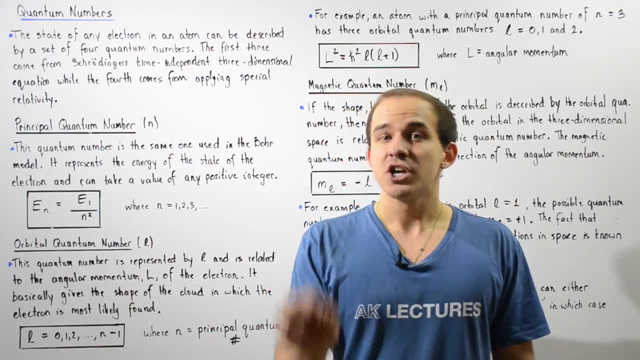 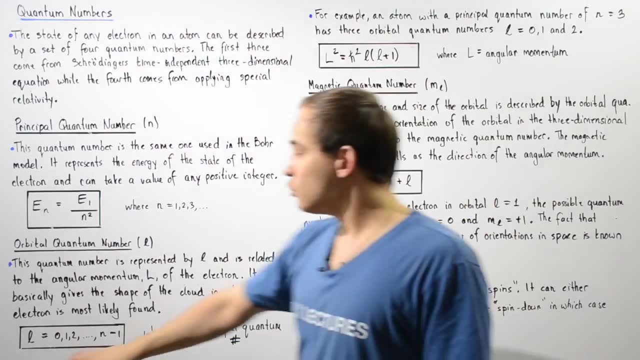 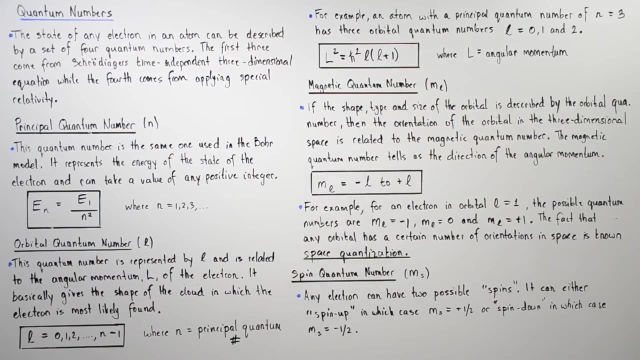 if we know that some given atom has three principal quantum numbers, so n is equal to 3, then that means, by the way, we can determine the number of orbitals that our atom has. So by using this equation we see that our atom has three different orbital quantum numbers. So 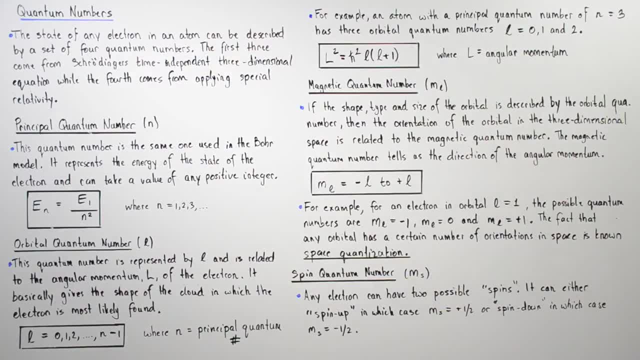 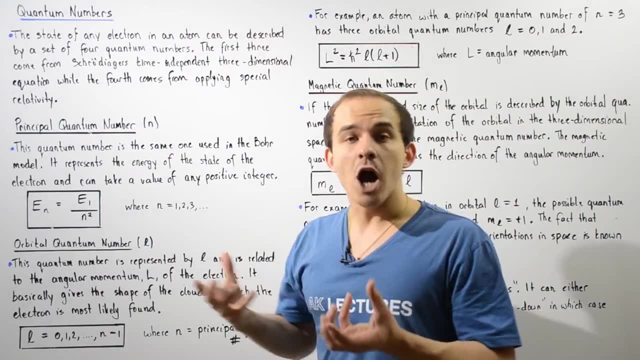 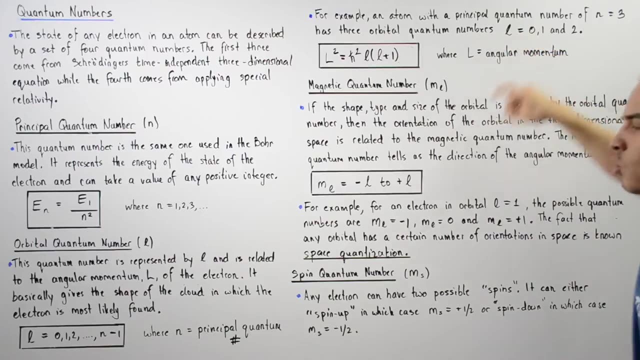 L can either be equal to 0,, 1, or 2,, where each one of these quantities represents its own shape and size and type of the orbital. the electron cloud that we are dealing with, For example, L equals 0, corresponds to a spherical electron cloud. So L is equal to 0,, 1,, 2,, 3,, 4, and all the way up to n minus 1,, where each one of these quantities represents its own shape and type of the orbital, the electron cloud that we are dealing with. So 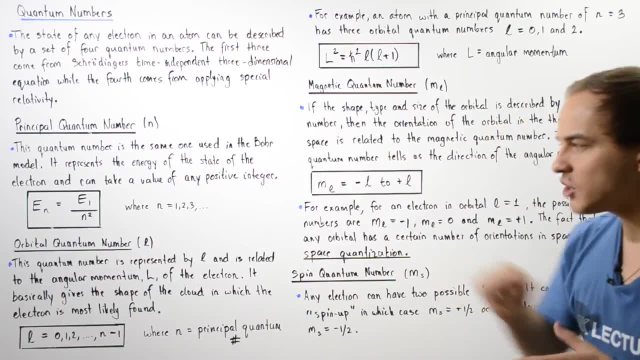 L equals 0 corresponds to a spherical electron cloud. So L equals 0 corresponds to a spherical orbital cloud. So L equals 0 corresponds to a spherical electron cloud. So L equals 0 corresponds to a spherical orbital, as we'll discuss in a future lecture. Now earlier we said that the 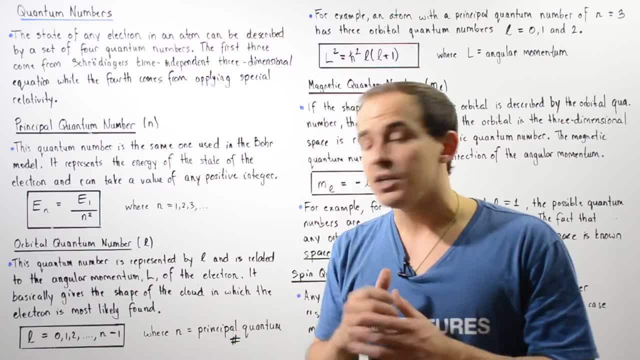 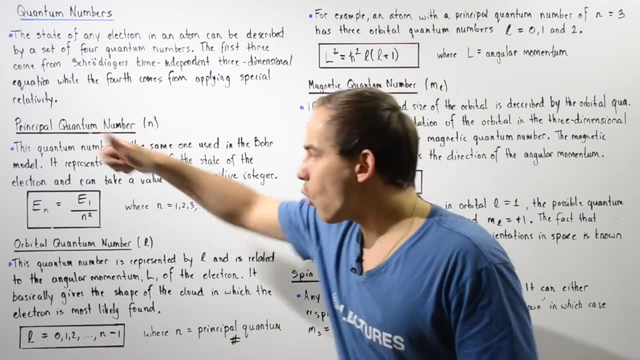 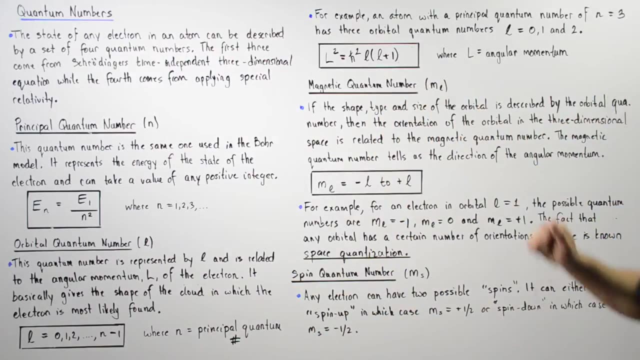 orbital quantum number is related to something known as the angular momentum of our electron. Now the relationship between the orbital quantum number L and the angular momentum given by uppercase L is given by this equation. So the angular momentum squared is equal to: 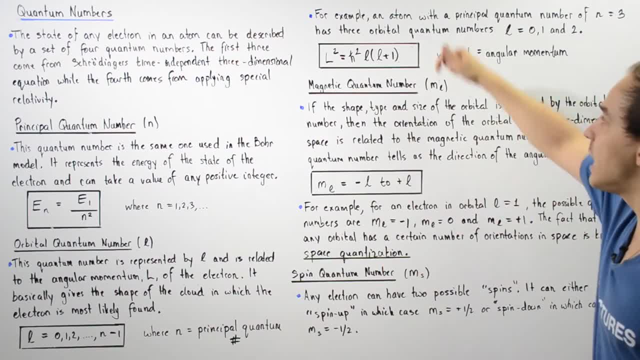 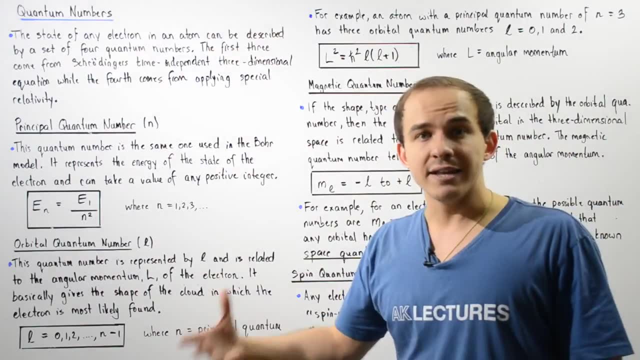 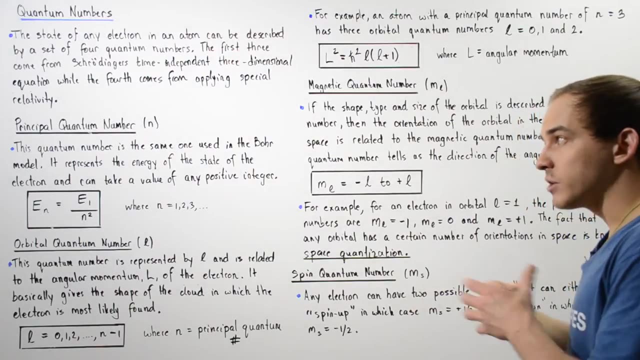 H bar squared, multiplied by L, multiplied by L plus one, where L is the orbital quantum number. H bar is a constant that is related to Planck's constant and L is the angular momentum. So we see a very important trend. Basically, the principal quantum number determines the 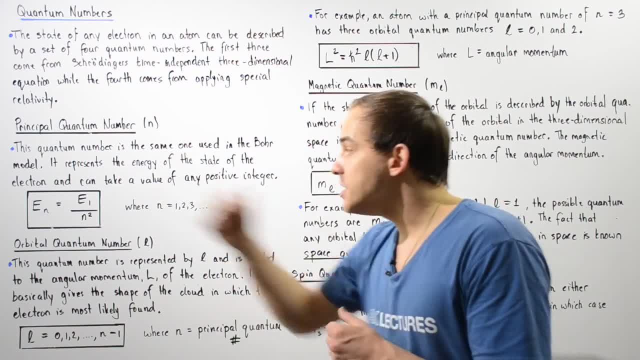 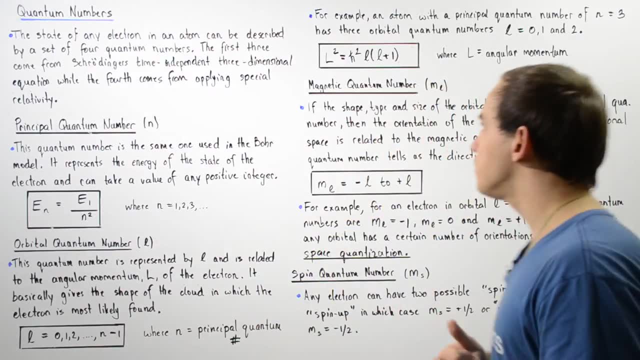 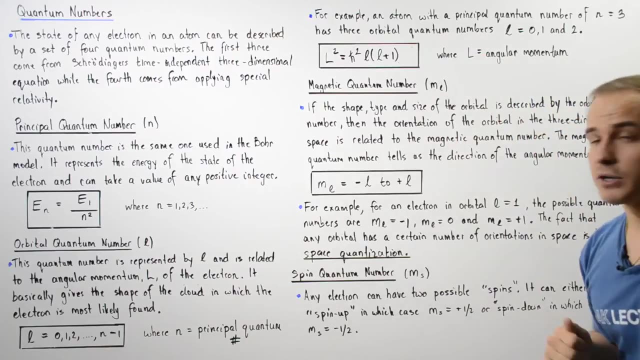 number of orbitals, we can have the number of orbital quantum numbers that any atom can can have. Now let's move on to the third quantum number we call the magnetic quantum number. that is given by M with the L subscript on the bottom. Now, if the shape, the size and the type of our 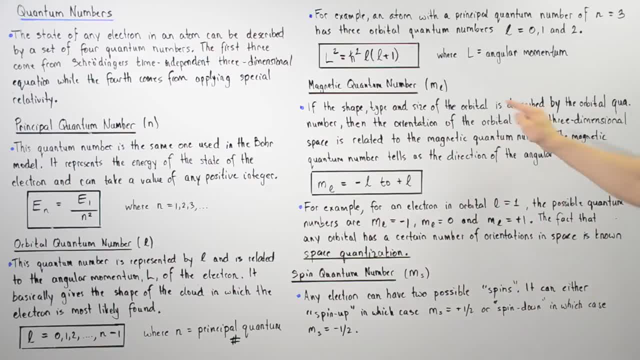 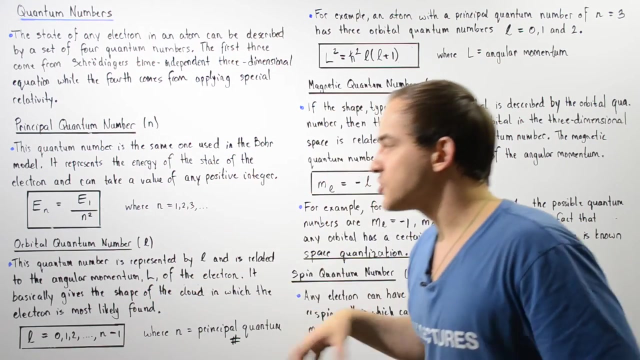 orbital, the electron cloud around the atom, is described by the orbital quantum number L. then the orientation and the direction of this orbital, the electron cloud, in the three-dimensional space, is given by the magnetic quantum number. So basically, the orbital quantum number describes. 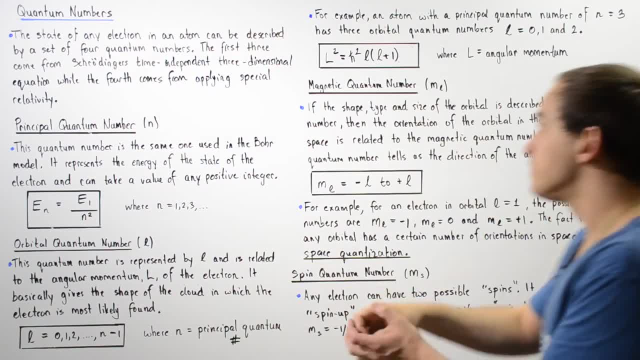 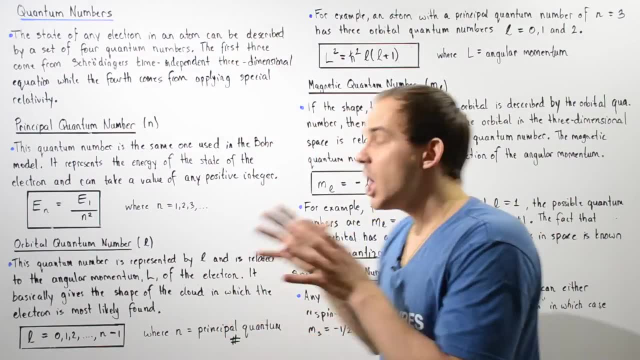 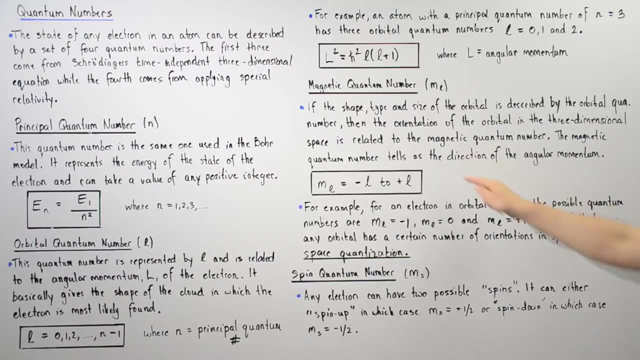 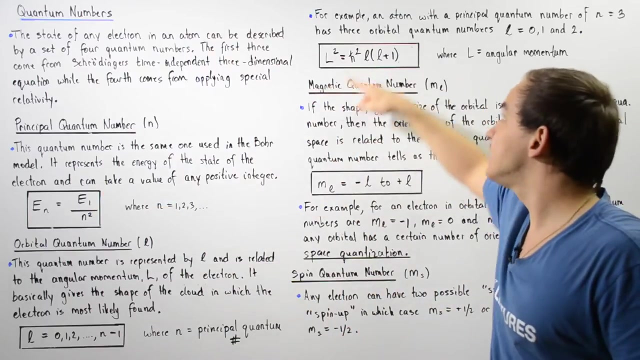 the type and the size and shape of our orbital, but the magnetic quantum number designates the orientation and direction of our orbital in the three-dimensional space. So the magnetic quantum number tells us the direction of the angular momentum, while the orbital quantum number describes the magnitude of our angular momentum. Now, what exactly are? 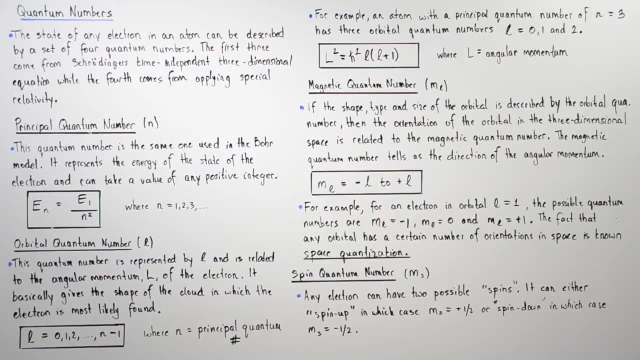 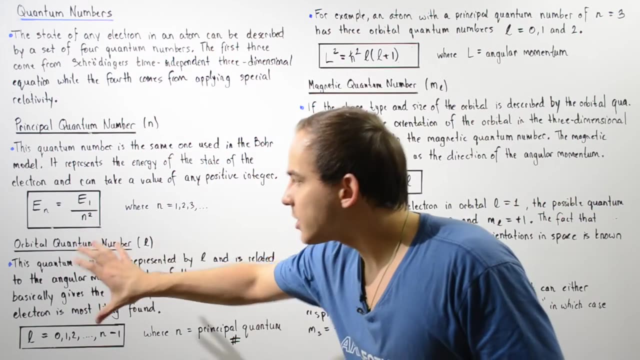 the values that the magnetic quantum number can take. So, basically, this is the equation that tells us the different values that the magnetic quantum number can take. So, in the same way that the principle quantum number determined the number of orbital quantum numbers, the orbital quantum 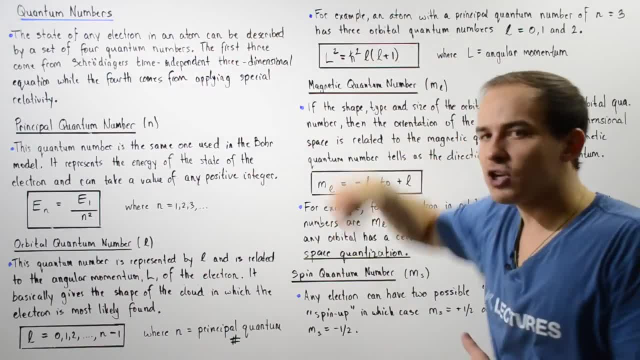 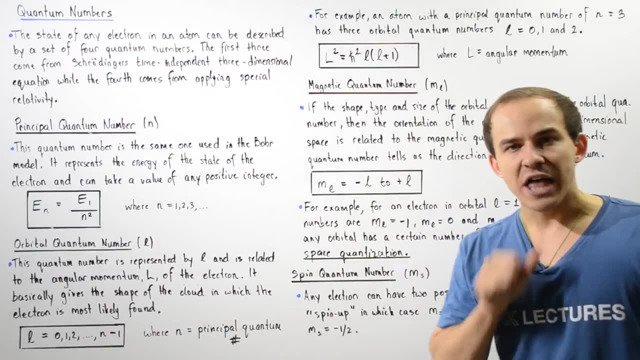 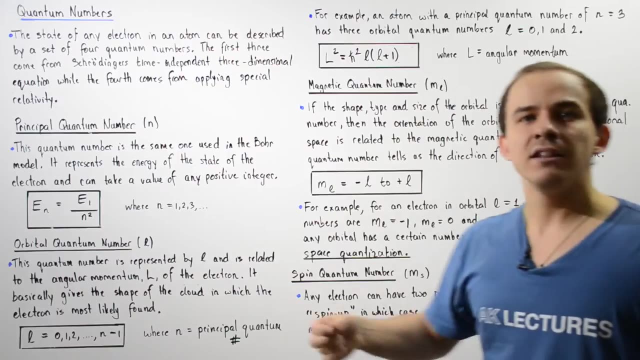 numbers determines the number of magnetic quantum numbers. So ML is equal to negative L to positive L. So to see what that means, let's suppose that, for example, an electron is found within orbital L equals one. So because we know what the orbital quantum number actually. 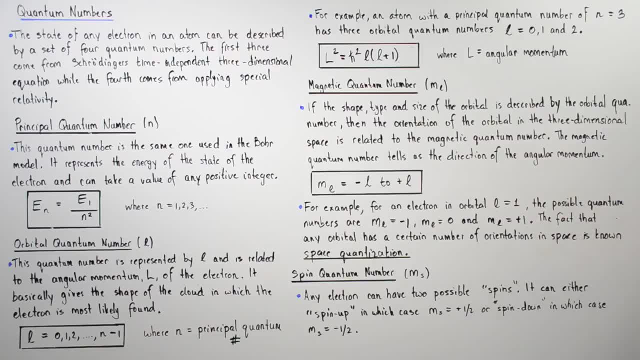 or whole alternative value. we very quickly leave it behind and we take the form of the L to the power of the electron, of which we're finding the magnitude. electrons help us is because L is equal to one. we know that the possible magnetic quantum numbers are negative L. 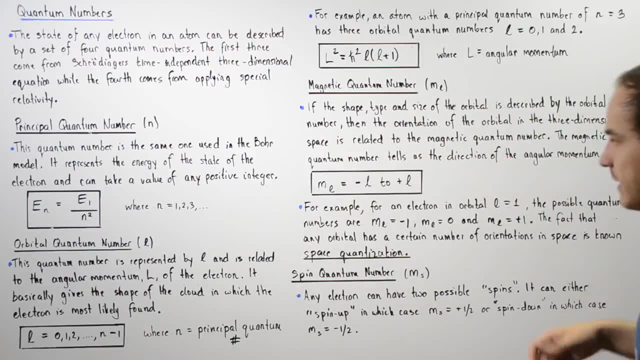 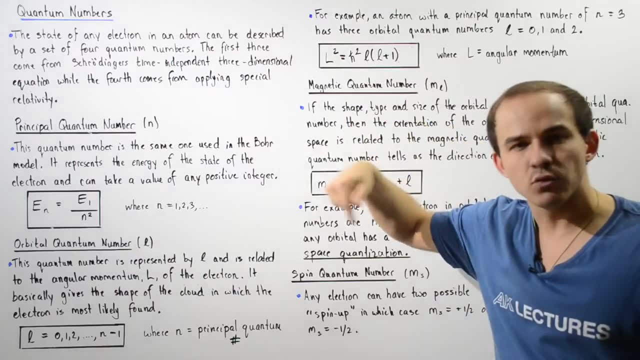 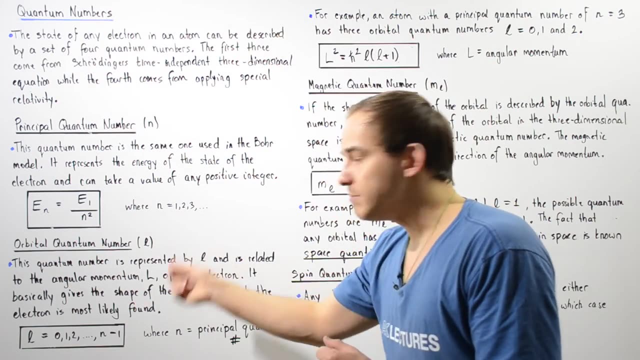 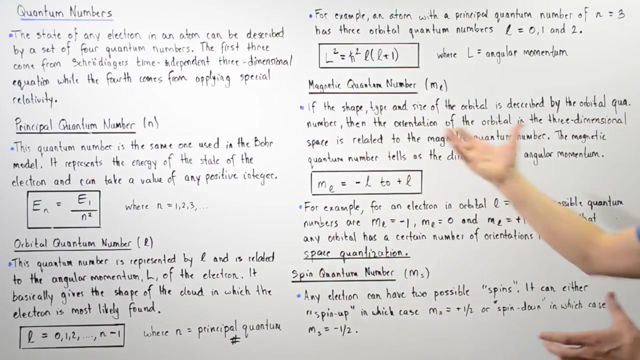 zero and positive L. So basically, if L is equal to two, then our ML can be negative two, negative one, zero, positive one and positive two. So we see that for any given orbital quantum number, L, there is a certain specific number, a certain limit to how many magnetic quantum numbers. 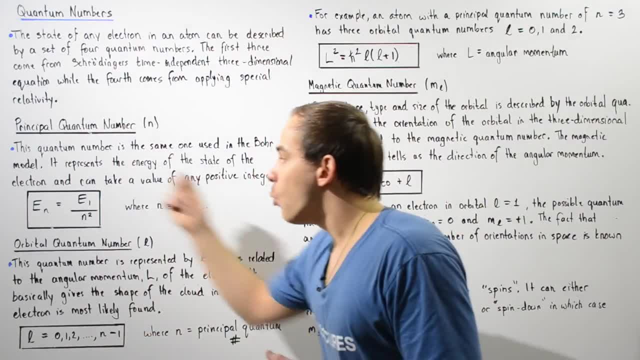 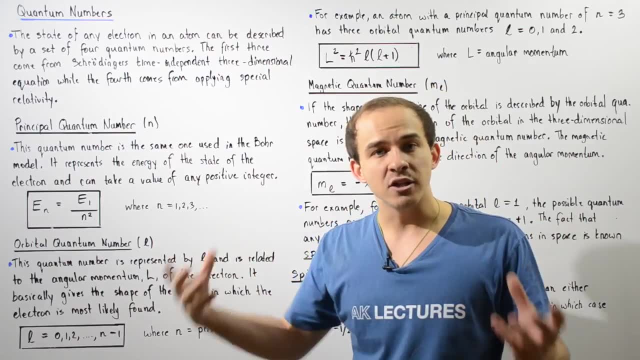 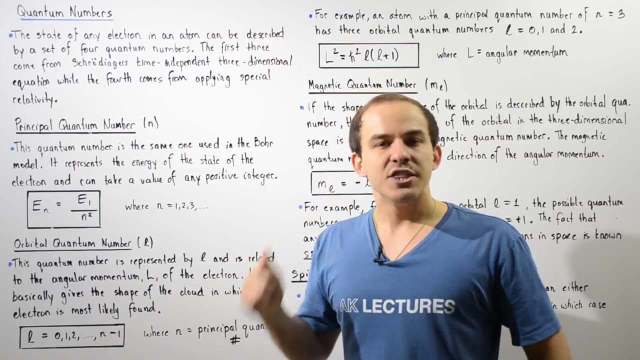 there are. That is, if we know what the orbital quantum number is, if we know what the shape of that orbital is, if we know what the shape of the electron cloud is, then we know there is a limit to the number of orientations that this orbital can take. this orbit can take. 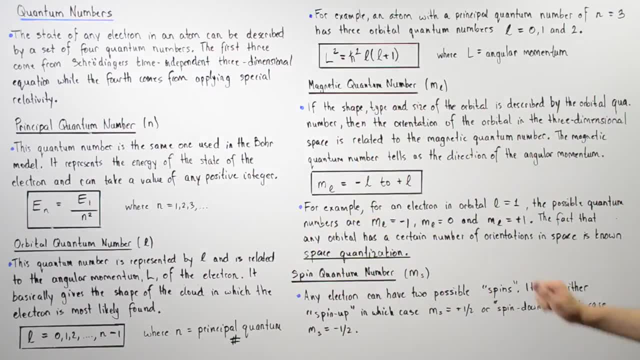 within the three dimensions. So, for example, for L equals one, there are three different orientations and this is known as the space quantization of the magnetic quantum number. So basically, the fact that any given orbital has a certain number of orientations has a limit to the number of orientations it can take. 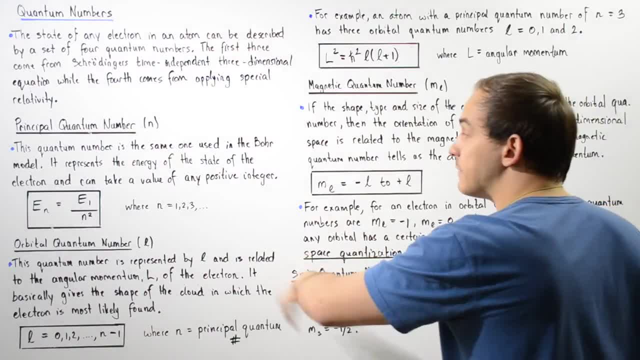 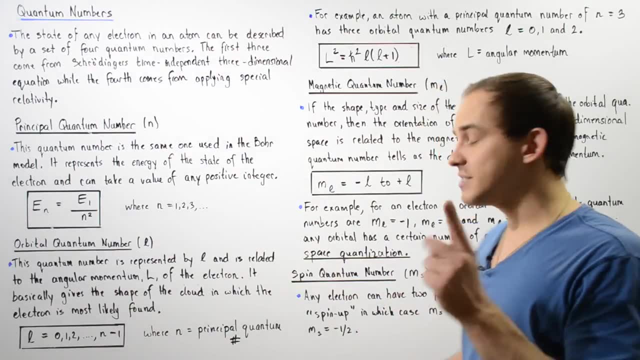 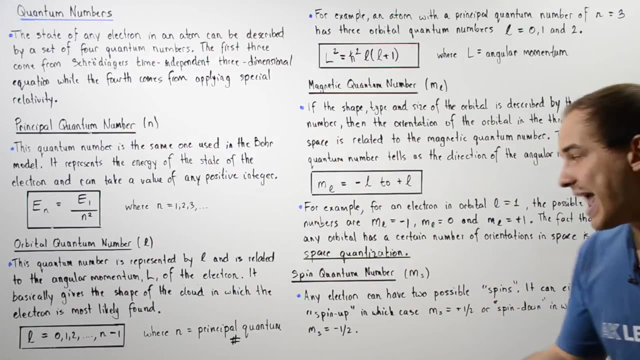 this is known as space quantization. And finally, the last and fourth quantum number is known as the spin quantum number and this is given by M with the S subscript. Now, basically, any one electron within any given orbit can have one of two possible. 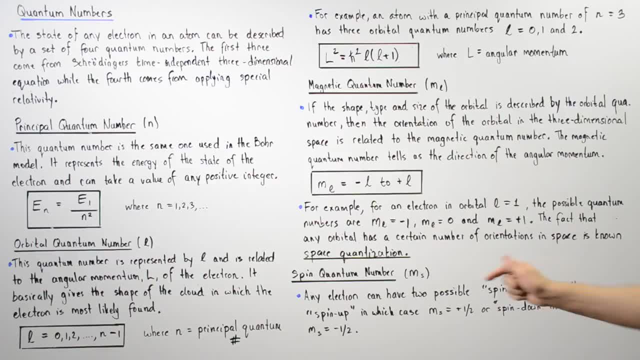 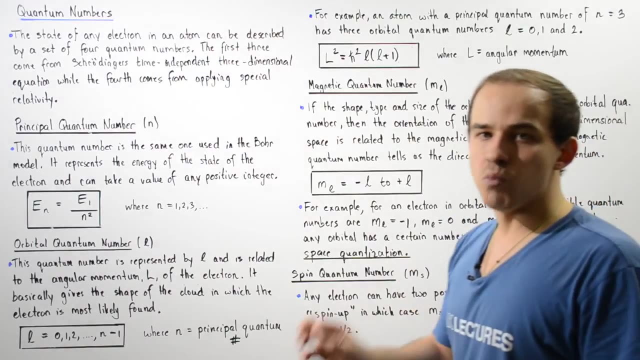 spin numbers. So any electron can have two possible spins. It can either have a spin up, in which case the MS is equal to positive one half, or it can have a spin down, in which it and ms that is equal to negative one half. Now, in a future lecture we're going to discuss 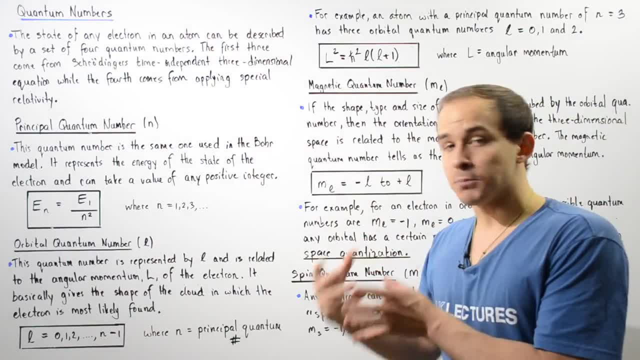 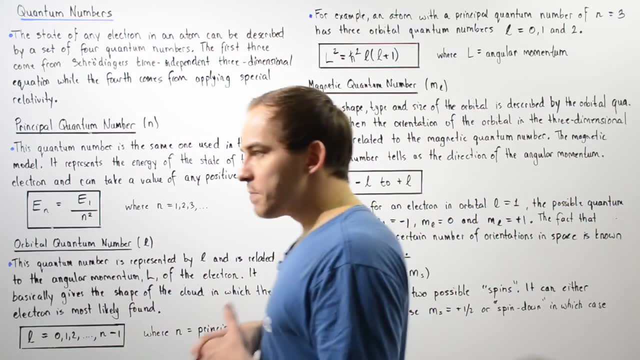 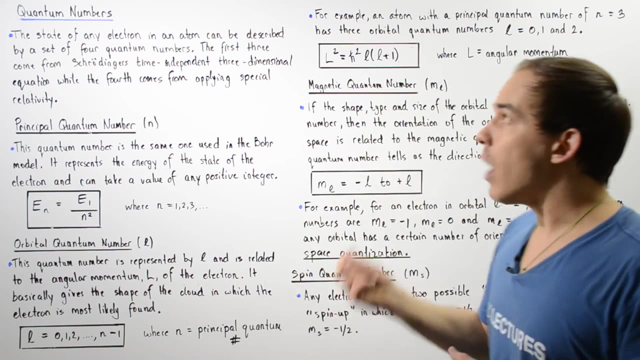 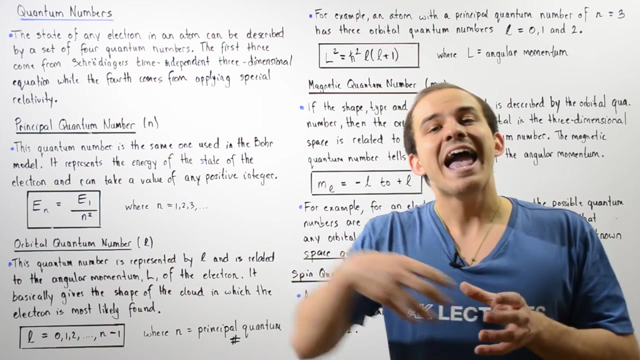 this spin quantum number and its interpretation in more detail. So what exactly is the quantum number? So, basically, any electron within any given atom can be described by using four unique quantum numbers, A set of four quantum numbers. The principal quantum number tells us the energy. 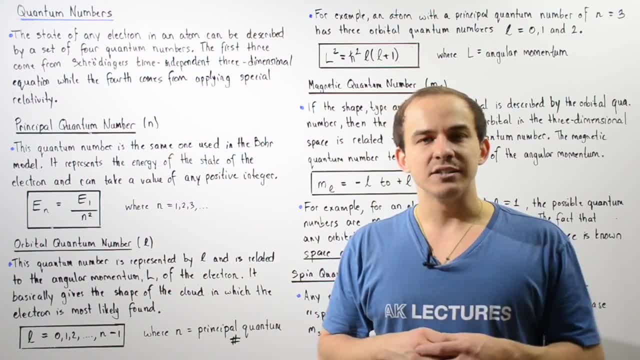 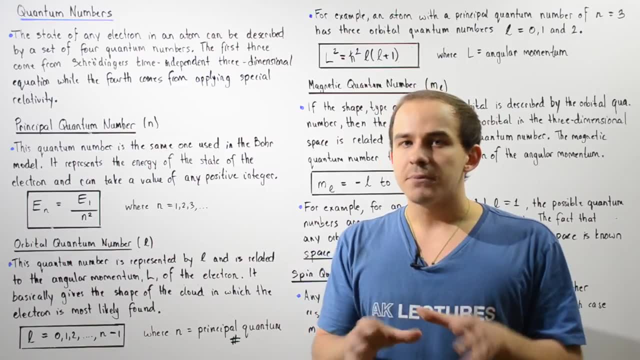 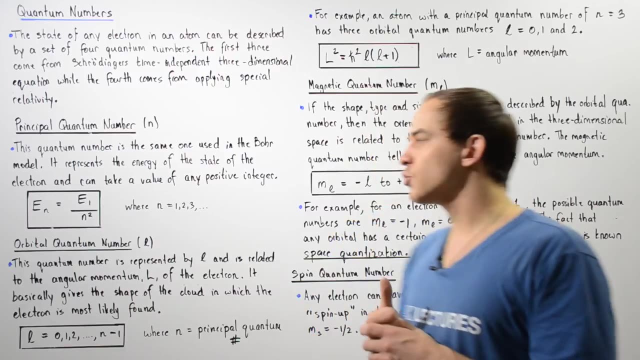 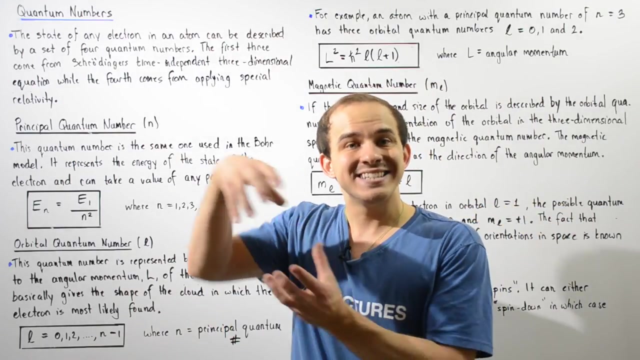 level of our electron. The orbital quantum number tells us the shape of that electron cloud, also known as the orbital. Remember, the electron cloud designates the probability of finding our electron within that specific region of space around our atom. The magnetic quantum number tells us the shape and the orientation of that orbital in three-dimensional space. and 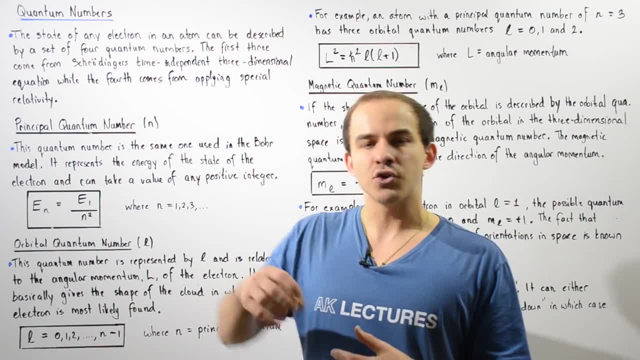 the spin quantum number tells us if our electron is spinning up or spinning down. 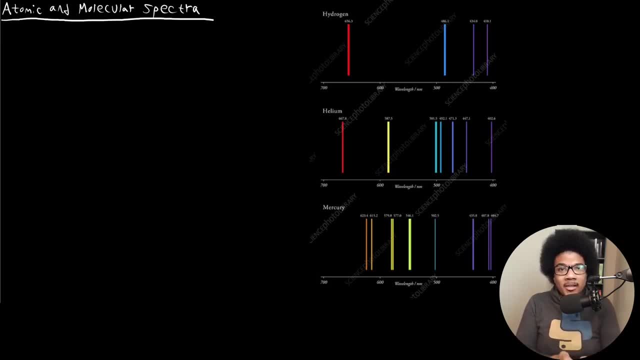 In this video we're going to talk about atomic and molecular spectra. Now, when I first introduced this course, I noted that it's going to be a focus on quantum mechanics and spectroscopy. right Now, spectroscopy is the second piece of this, And now that we've talked about quantum,